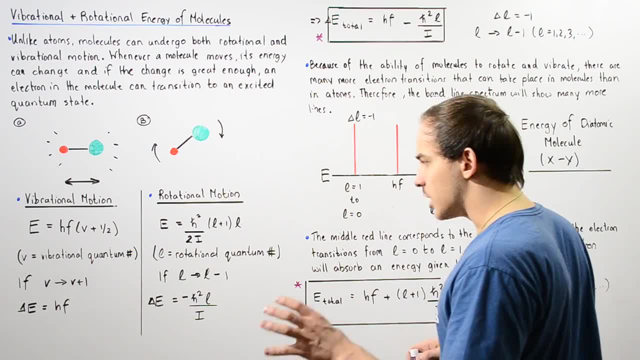 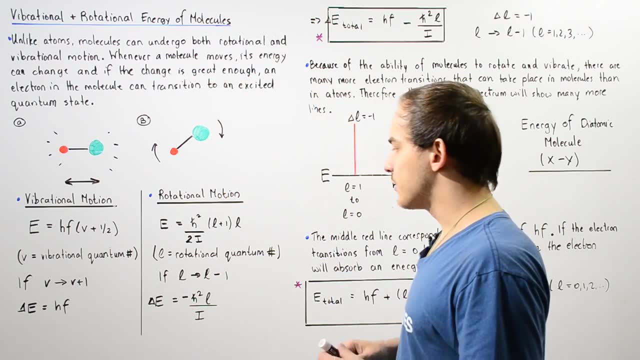 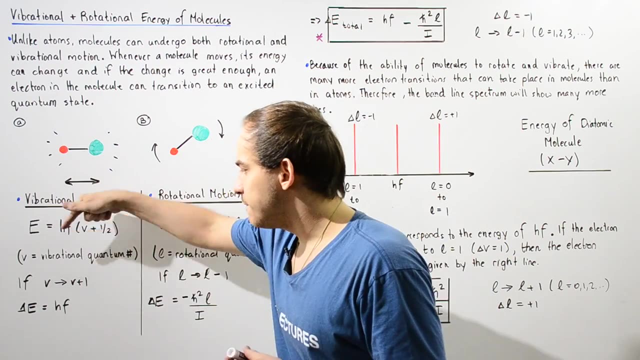 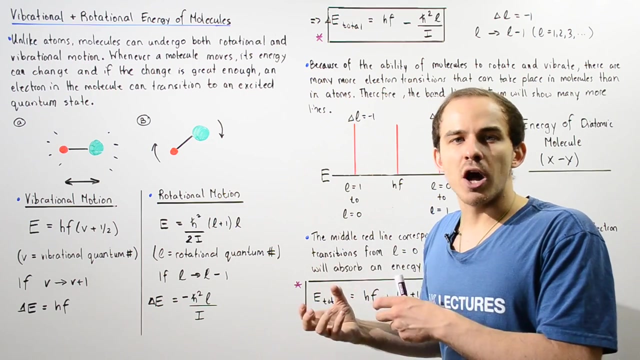 one multiplied by L, where L is the rotational or angular quantum number. So L is also a number that begins with zero and increases by increments of one. Now let's suppose our electron transitions from V to V plus one and from L to L minus one. In such a transition the electron is said to gain. 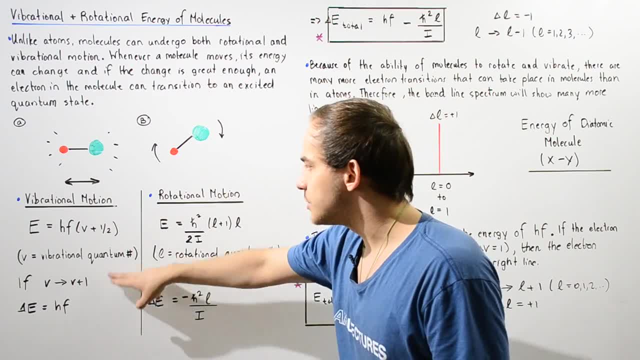 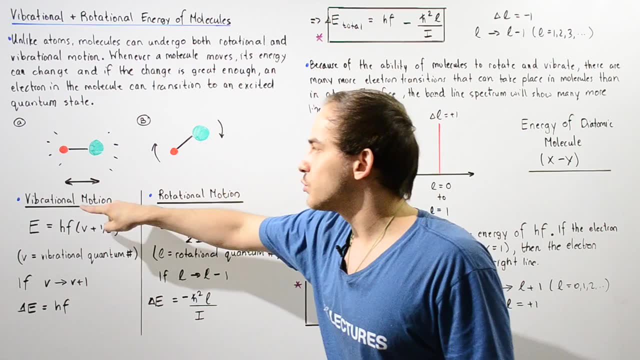 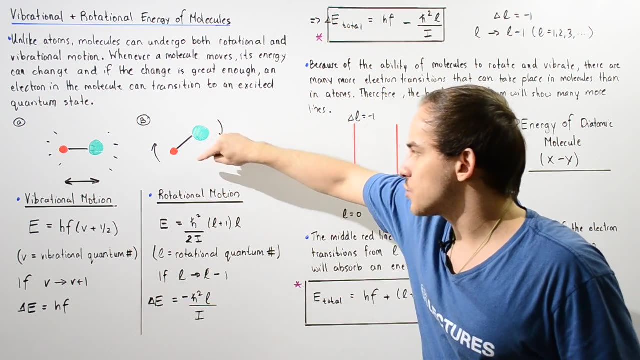 energy. And if we use these conditions and these equations, we see that, for such a transition, our change in energy as a result of the change in vibrational motion is given by this equation, while our change in energy as a result of the rotational motion. 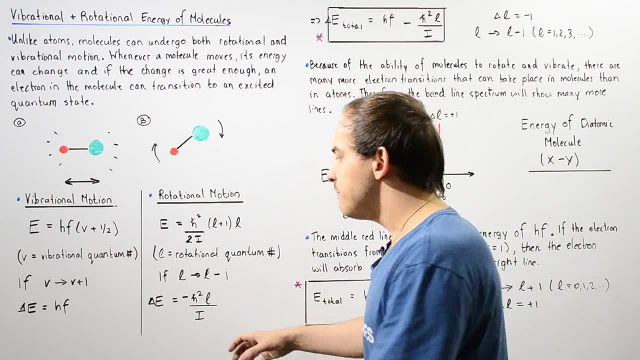 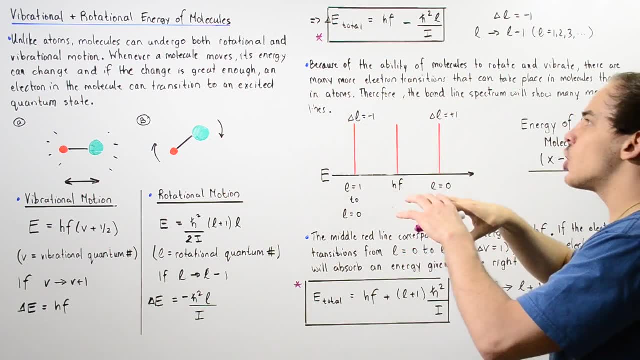 is given by this equation. So we have a change in energy as a result of the rotational motion given by this equation. now if we combine these energies, that will give us the change in energy total. so the total change in energy of our diatomic molecule as a result of the change in vibrational 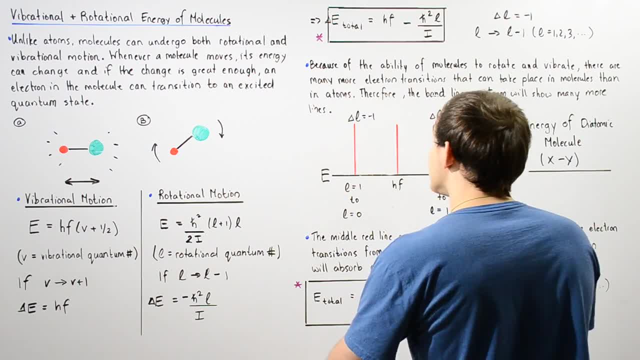 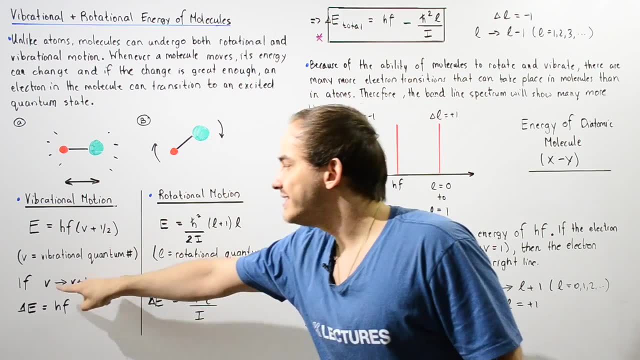 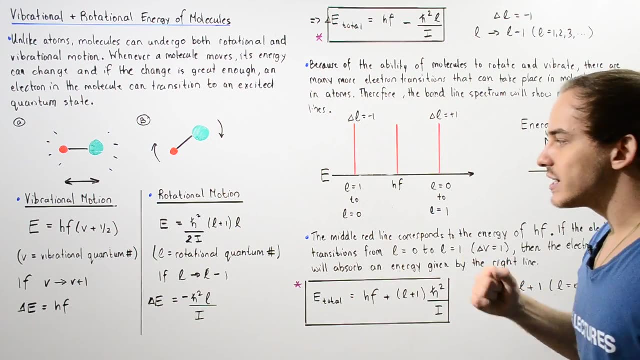 and change in rotational motion, and that is given by the following equation. so this equation is true as long as the delta v is positive one, so the electron jumps from v to v plus one, and as long as the delta l is negative one, so l jumps. or the electron jumps from l to l minus one, where l 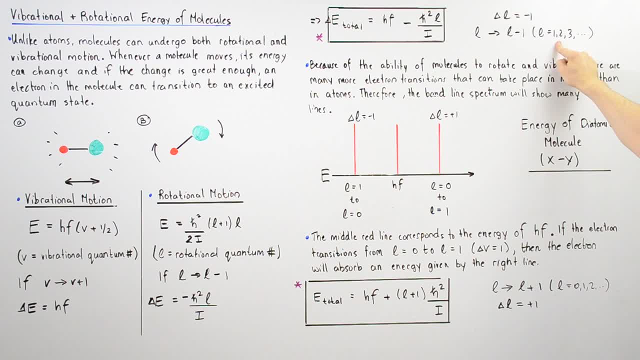 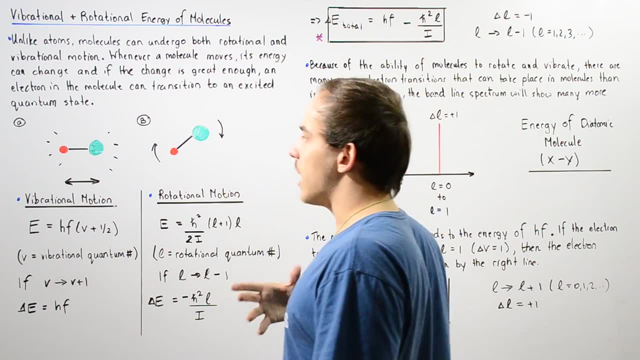 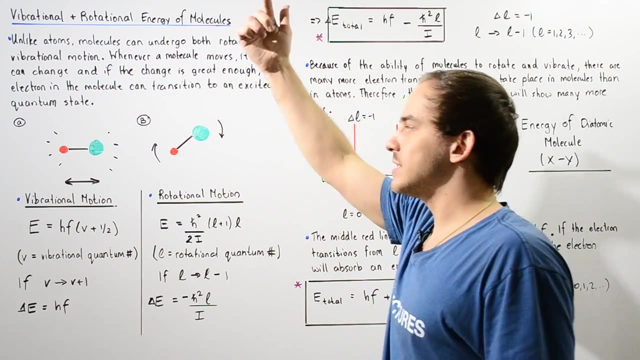 in this case is a number that begins with one and goes to two, to three, to four and so on. so this is our equation that gives us the change in energy of our molecule, and if the change is greater than one, then there is a momentary shift to the external rotation of our molecule, as we graphs figure here. 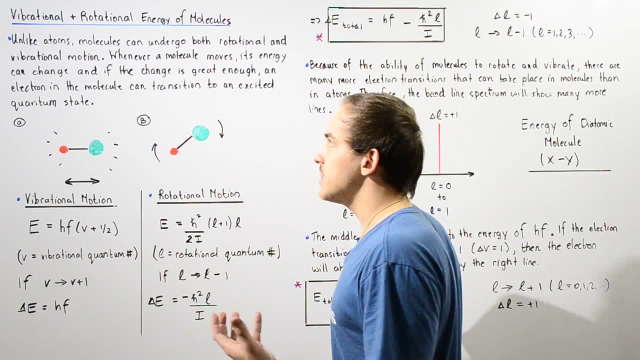 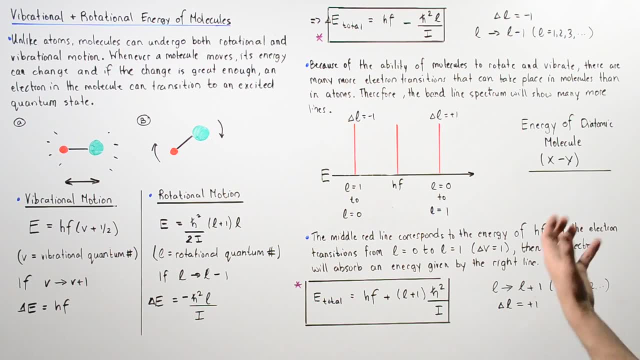 that pb is actually equal to zero pean, that this my can. additional weight. questioned w, if I can eventually measure this moment that I've overlaid this equation into the vedic system. so I think that pr very critical for me to figure out what to do or to why that isuse great enough. 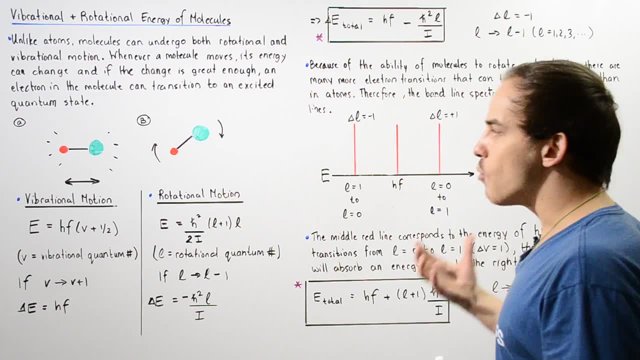 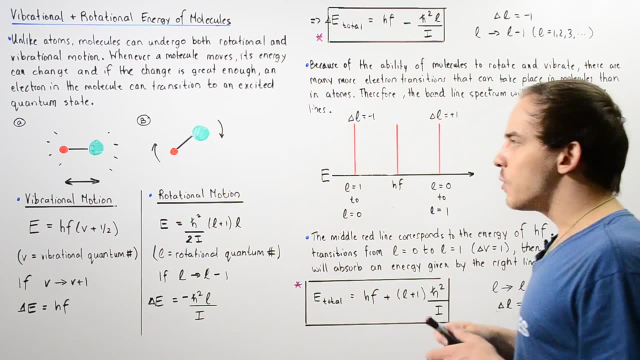 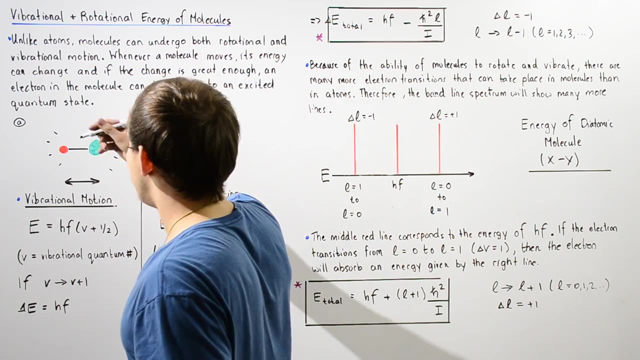 the electron can actually gain that energy and transition from a lower to higher state, many more lines for the molecules than for our individual constituent atoms. So let's suppose we take some particular diatomic molecule. So our red is given by, let's suppose, X and our Y. 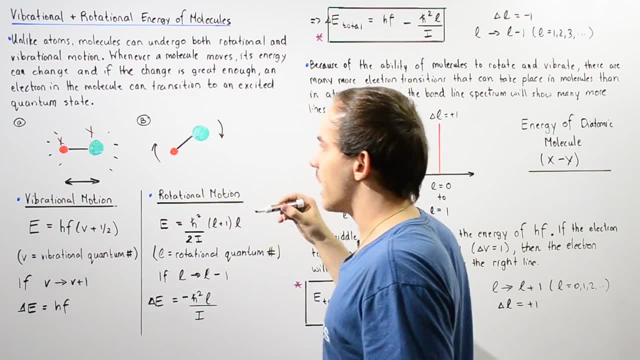 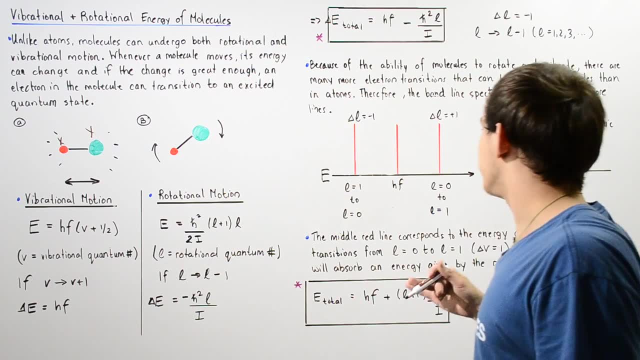 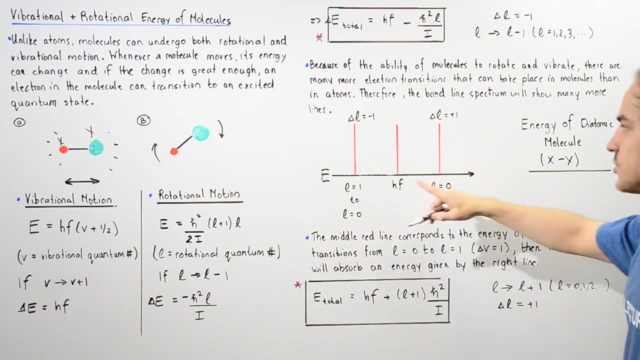 and our green molecule, atom, is given by Y. So X can be, for example, H and Y can be Cl. So we're examining, let's suppose, a hydrochloric, a hydrochloride molecule. So we basically have the X axis, which is our energy, And as we go from this side to this side, our energy increases. 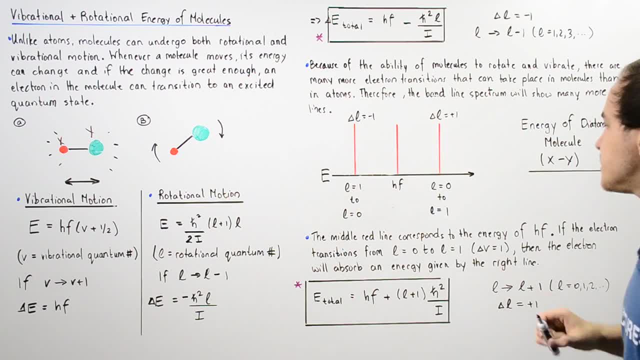 Now the middle line. the middle red line corresponds to the energy of H multiplied by F. Now what exactly is our right line? So the third line from this side. So this basically corresponds to a delta L of positive one. So that means, if the L transitions, 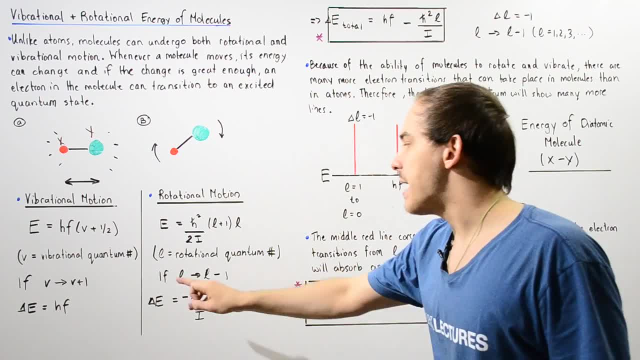 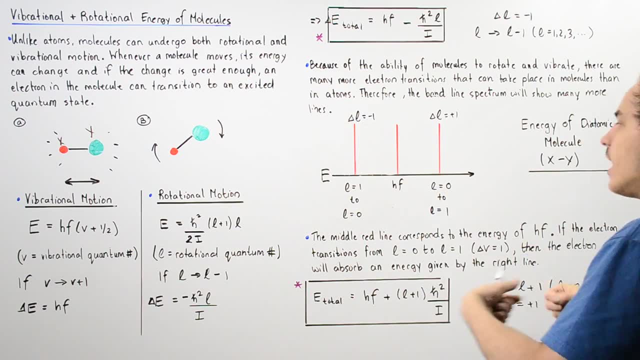 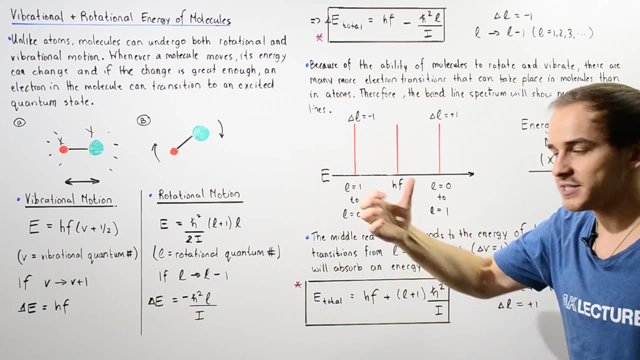 not from L to L minus one, but from L to L plus one. then our atom, then our molecule and electron will gain a certain amount of energy and it will jump from this state to this state And notice that for this particular case our formula is not given by the delta L of positive one. 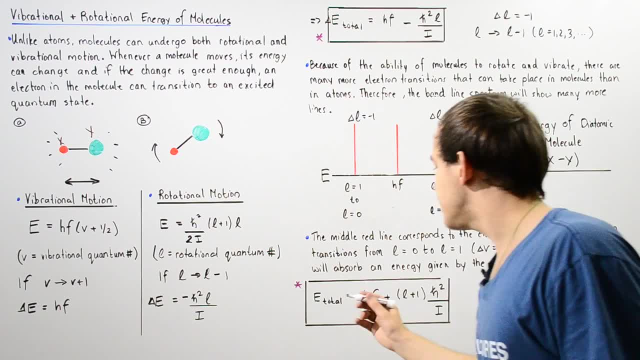 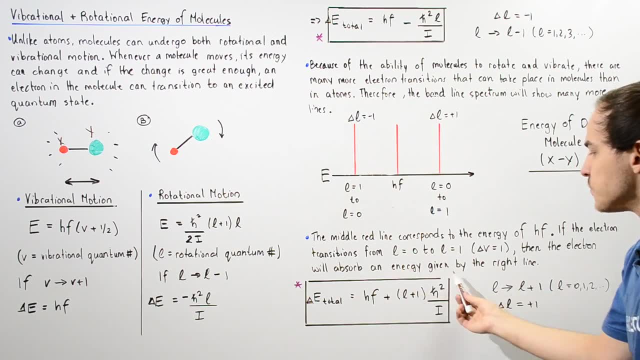 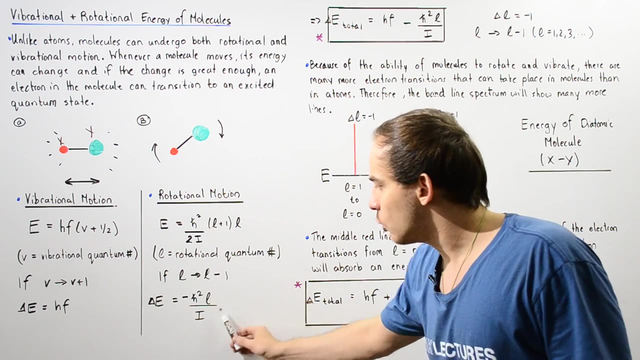 it's given by this equation, but it's given by this equation. So basically, the delta E total is given by HF plus this quantity, where this quantity comes from, using L to L plus one. So our equation is no longer given by this, but given by this Now, because the V still goes from. 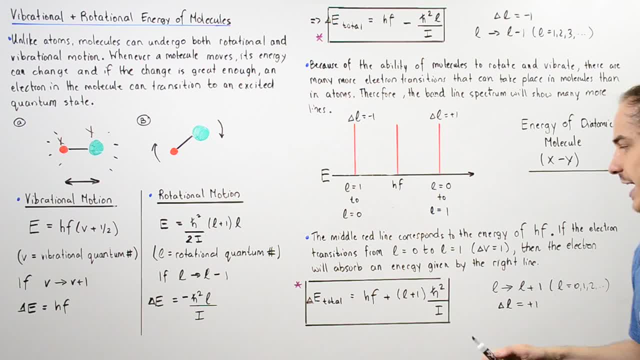 V to V plus one, the HF doesn't actually change. So this equation works as long as our delta V is still positive one and delta L is positive one as well, where in this case our delta L was negative one. So this first line basically corresponds to our electron absorbing. 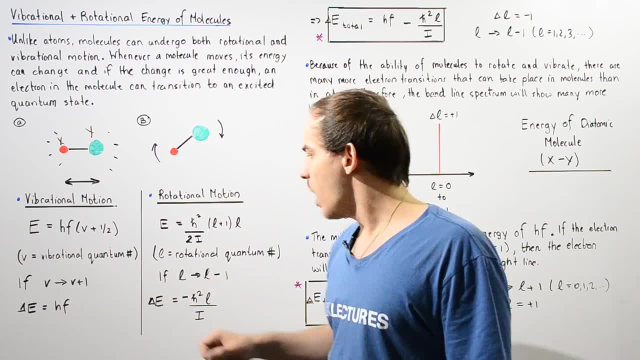 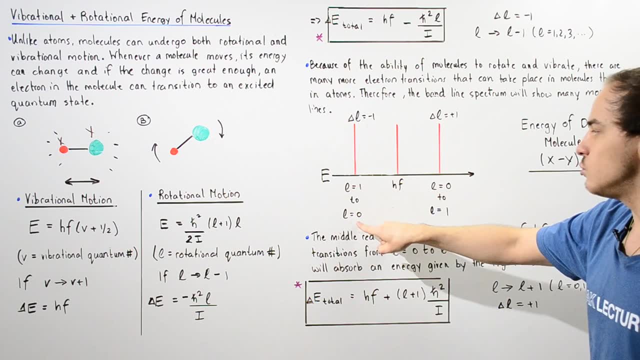 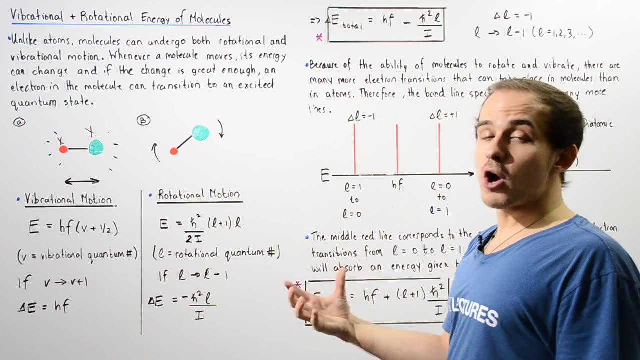 energy and jumping from V to V plus one and jumping from L to L minus one. So this line corresponds to L equals one to L equals zero, and this corresponds to on l equals zero to L equals 1.. And in both cases the electron is said to gain some photon of energy that has